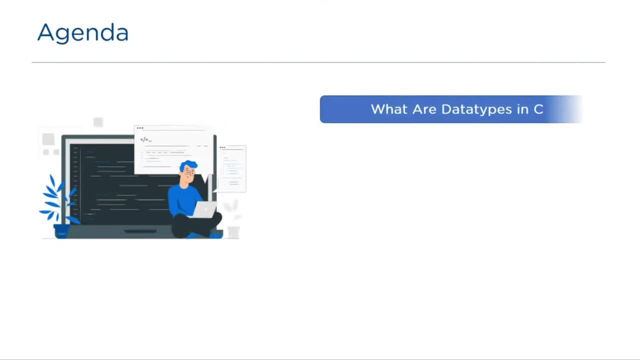 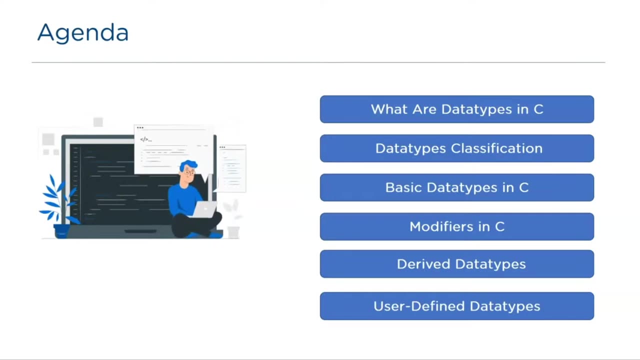 an update from us Without further ado. let's get started with the agenda for today's session. First, we will start by understanding what data types in C are. Next is the classification of data types, After that the basic data types and the modifiers, And finally the 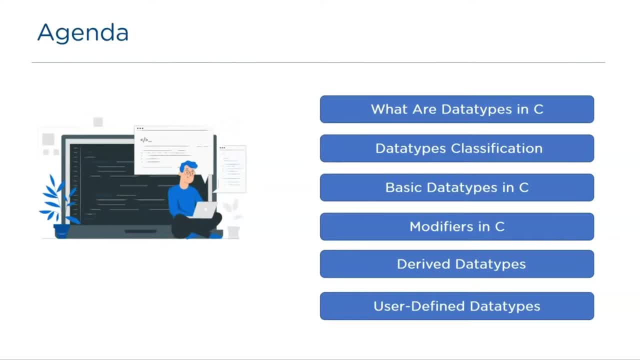 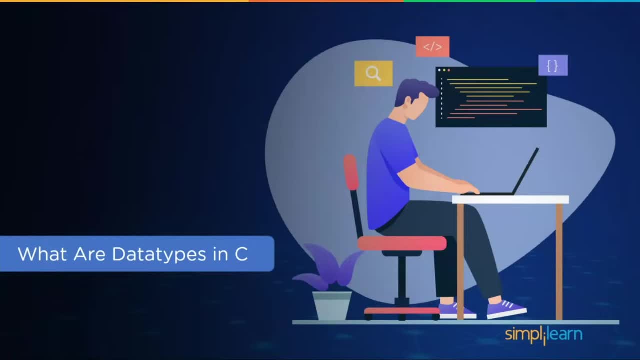 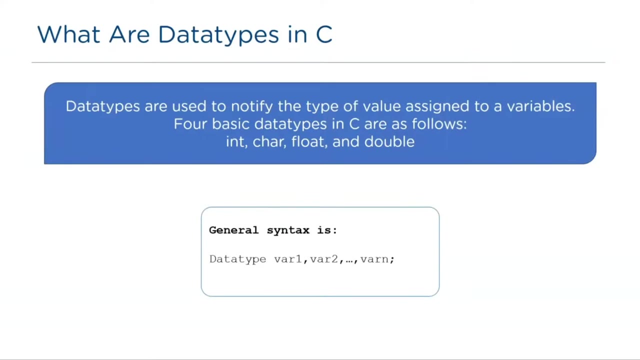 derived and user-defined data types in C. So I hope I have made myself clear with the agenda and we are good to get started Now. let's begin with. what are data types in C? Data types are used to notify the type of 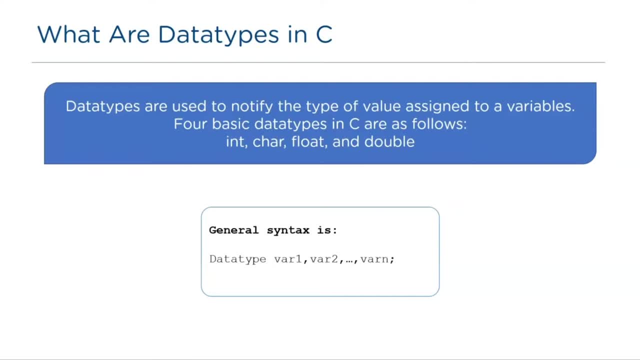 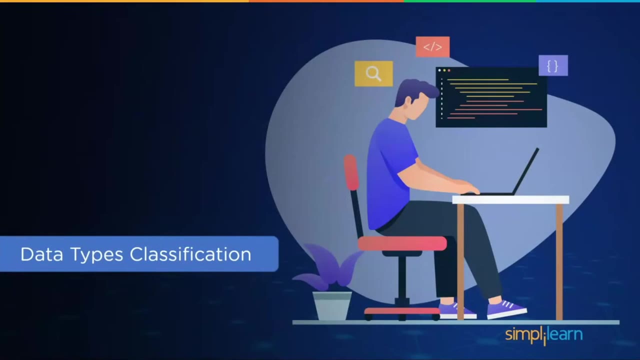 value assigned to a variable. Four basic data types in C are int, float, char and double, And the general syntax of data type is datatype, variable, list and semicolon at the end. Great, now that we know what are data types in C. Now let us understand the classification. 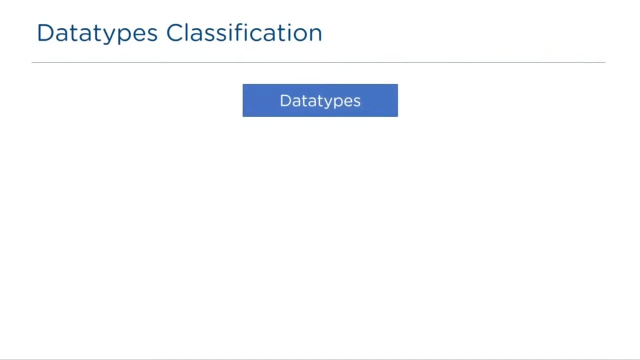 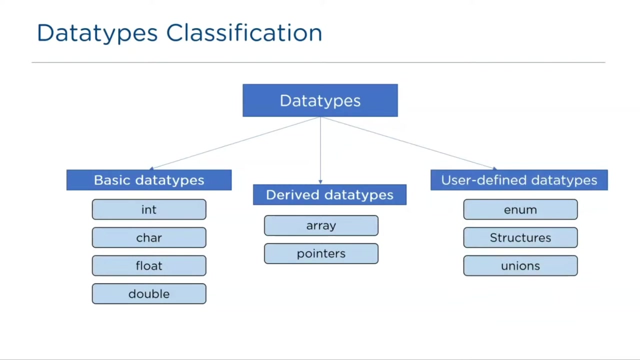 of data types. C data types are classified into three types. First up, we have basic data types, which are int, char, float and double. Then we have derived data types, in which we have arrays and pointers. And finally, user-defined data types, which are enum structure and. 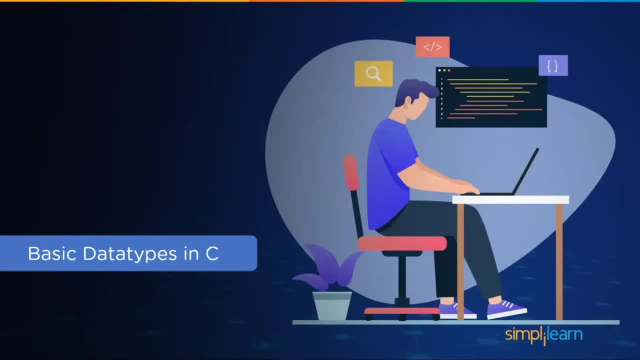 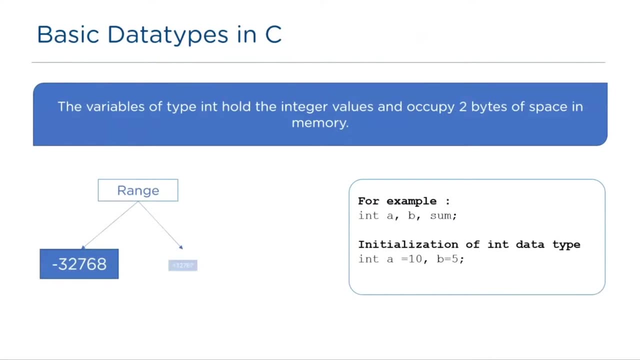 union. First let us understand four basic data types. in C, Variables of type int hold integer values ranging from negative 32768 to positive 32767.. And it occupies two bytes of memory size. In this example, a, b and sum are the variables. 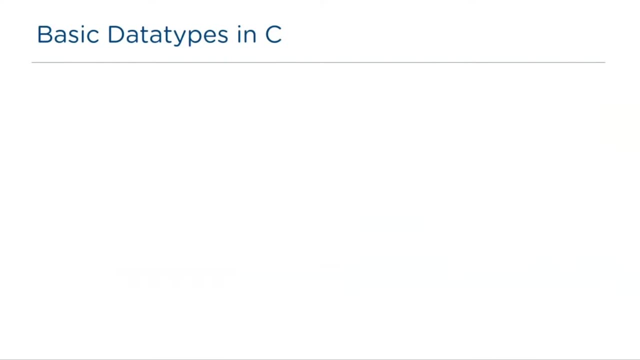 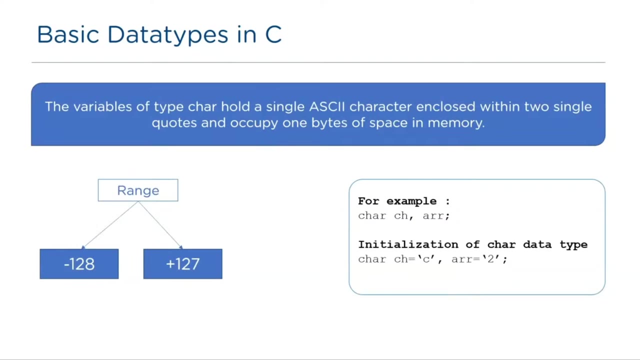 of type int that hold integer values. Next, the variables of type char hold a single ASCII character that contains numbers from 1 to 9, small and capital letters, e to z and some special characters, enclosed within two single quotes and occupies one byte of memory. 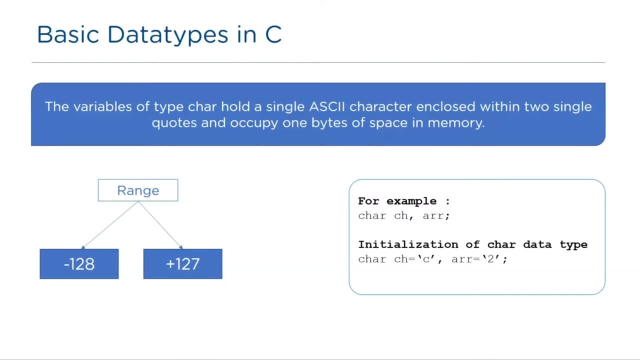 space. It ranges from negative 128 to positive 127.. The float data type variables occupy 4 bytes of memory space. that holds the value with decimal points. that is up to 6 decimal places. For example, pi and h are the variables of. 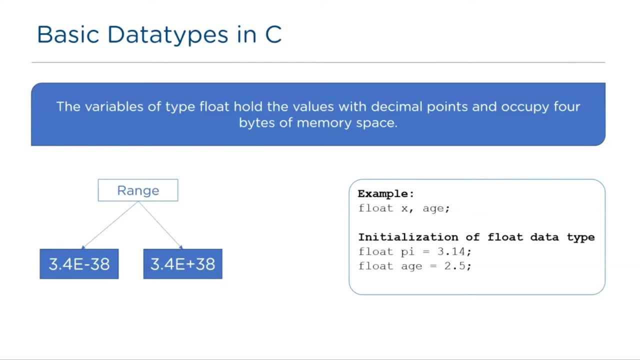 type float. they range from 3.4 into 10 to the power, of negative 38 to positive 30.. In The variables of type double hold values with decimal points and occupy 8 bytes of memory space. In this example, a is the variable of type double, ranging from 1.7 into 10 to the power. 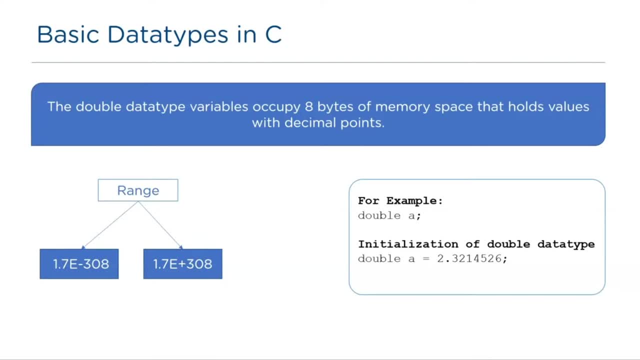 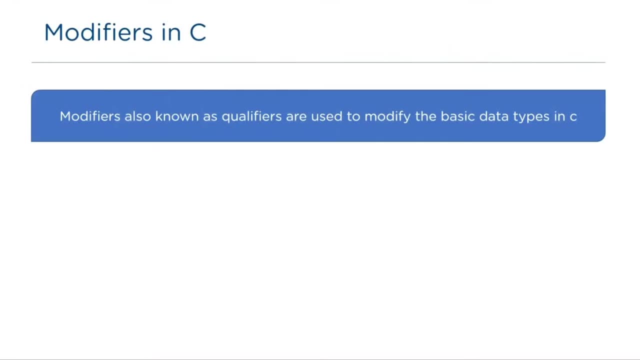 of negative 308 to positive 308.. Now let's have a look at the modifiers in C. Modifiers are also known as qualifiers, are used to modify the basic datatypes in C And the qualifiers are signed, unsigned, short and long. 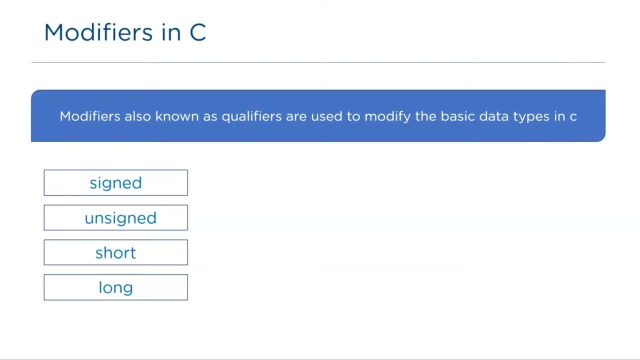 Signed modifiers are used to hold both negative and positive numbers At the same time. unsigned is used to store only negative numbers. So it's necessary to prefix the qualifier before the datatypes. And short requires memory space half the size of the basic datatype. 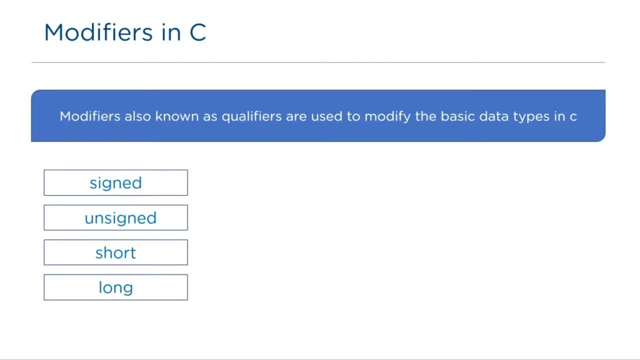 A long modifier is used to hold large numbers and it doubles the size of the datatype. The general syntax of handling modifiers is modifier, basic datatype, variable, list and semicolon. So in this particular example, unsigned is a modifier, int is a basic datatype and ye. 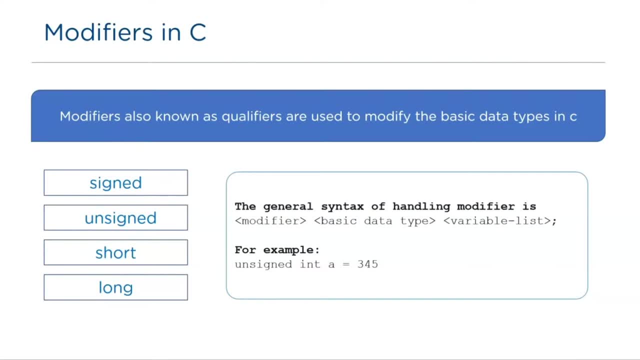 is a variable. We cannot apply qualifiers to the flow datatype, But we can increase the size of the double datatype by using a long qualifier. Also, we cannot apply qualifiers long and short on the char datatype. Not just this, There are also a wide variety of datatypes available in C programming language. 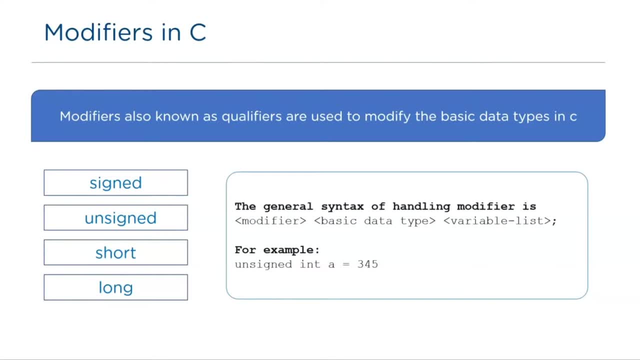 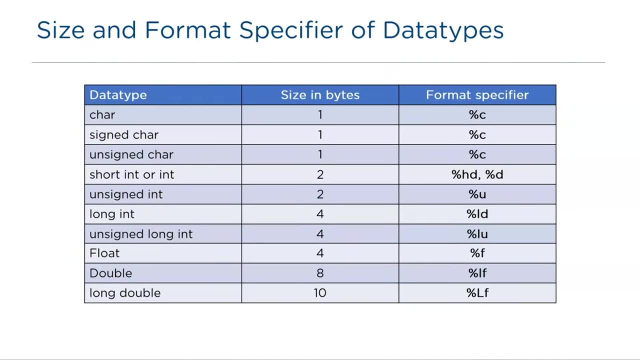 That comes in handy when you level up to the next stage with respect to your data. Let's look at the table that displays you the next range of datatypes and their format specifiers. You might wanna take a screenshot for future reference. Ok, 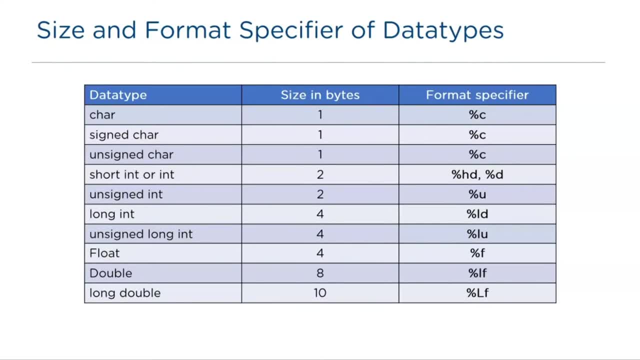 Let's get started with char For the datatypes char, signed char and unsigned char. the size is 1 byte and its format specifier is %c. Next int: The size is 2 bytes and its format specifier is %d. 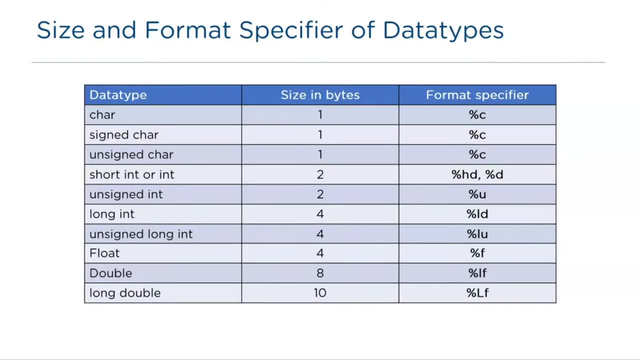 Unsigned int. the size is 2 bytes and its format specifier is %u. Next is long int. The size is 4 bytes and its format specifier is %ld. Unsigned long int. the size is 4 bytes and its format specifier is %lu. 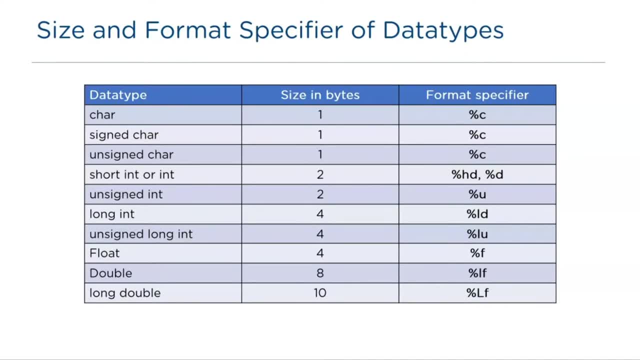 Next datatype is float, The size is 4 bytes and its format specifier is %f. Double the size is 8 bytes and its format specifier is %lf. Next, we have long. double the size is 10 bytes and its format specifier is %lf. 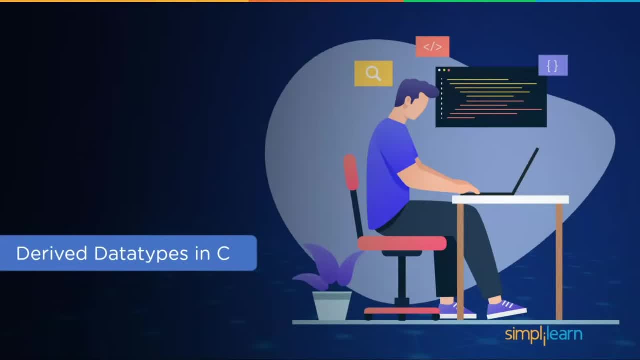 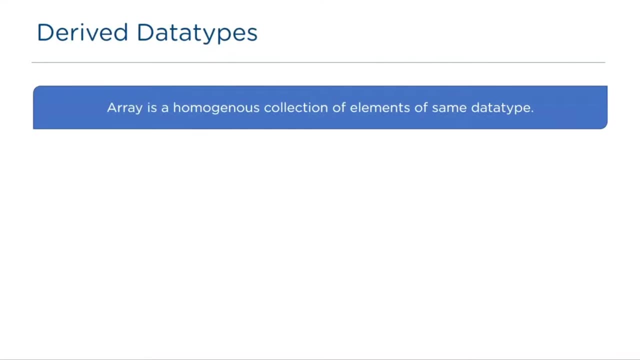 Now let's have a look at derived datatypes. As discussed earlier, array and pointers fall under derived datatypes. The array is a collection of elements of the same datatype, And that can be of int, float, char and double datatypes. 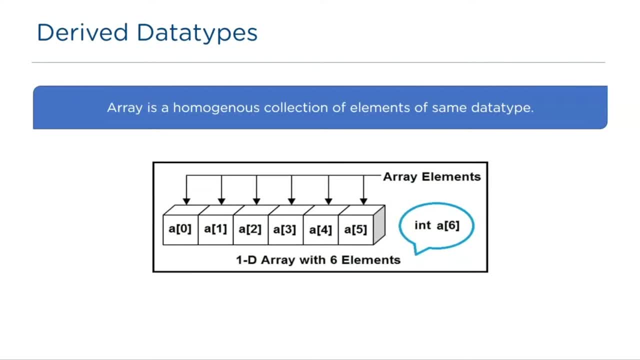 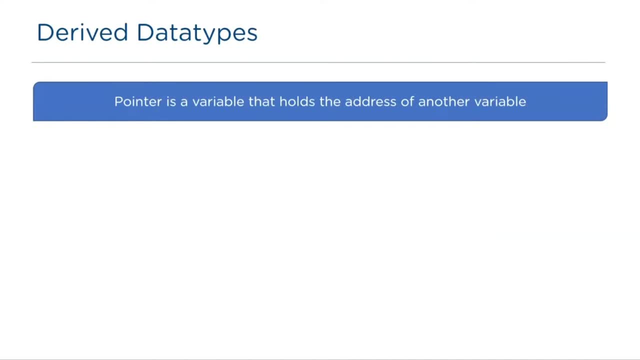 As you all can see, in this example the array stores 6 elements of the same type: int. Next, a pointer is a variable that holds the address of another variable declared under any basic datatype. In this example, the pointer variable holds the address of normal variables, in which the 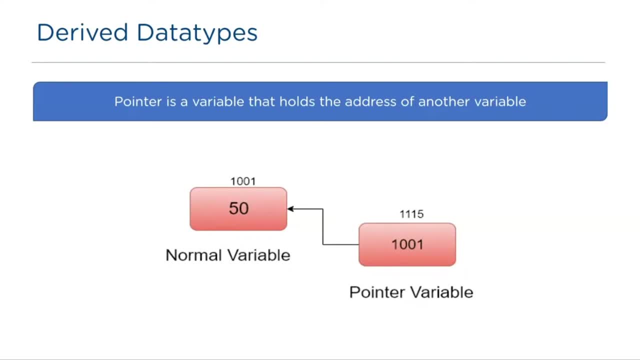 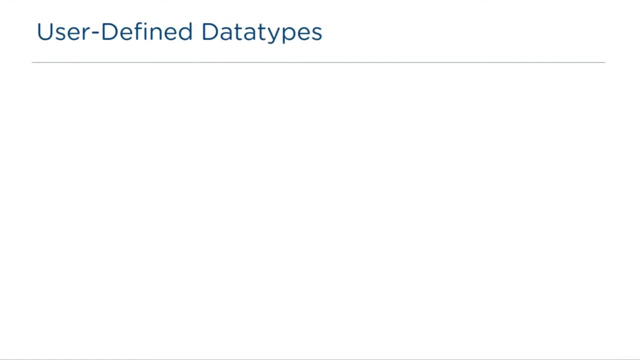 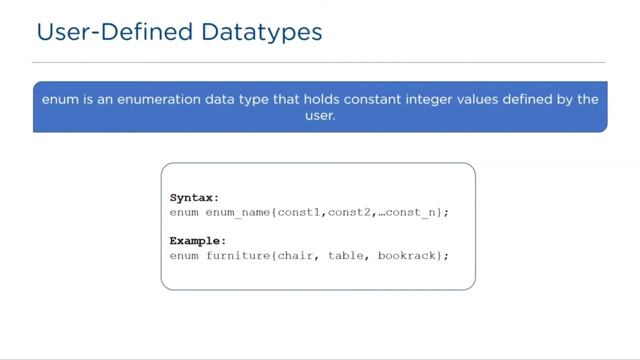 value 50 is stored. So I think you got a good understanding. Ok, so let us now understand user defined datatypes in C. Enum is an enumeration datatype that holds constant integer values defined by the user. The syntax of enum datatype is: enum, enum name and list of constant. 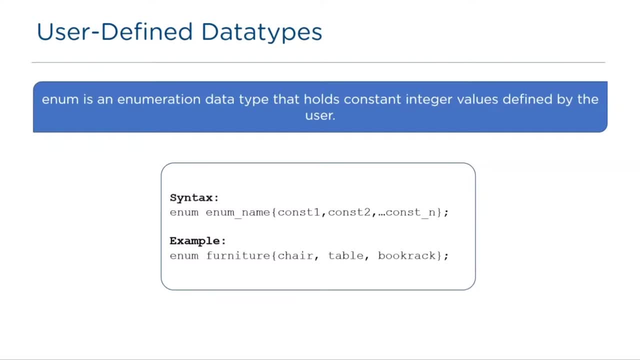 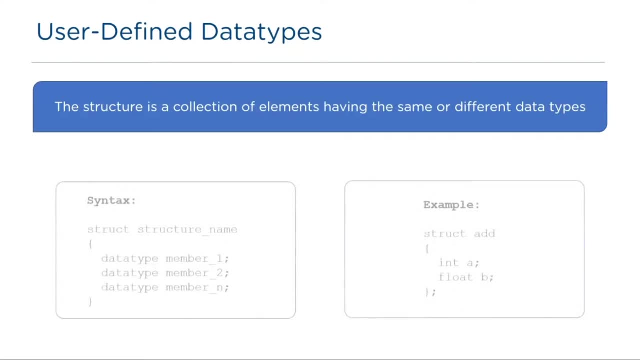 In this particular example, enum is a keyword, furniture as enum name and chair, table, book, rack would be constants. Next, The structure is a collection of elements having same or different datatypes. As you can see in this example, the elements declared as struct are of different datatypes. 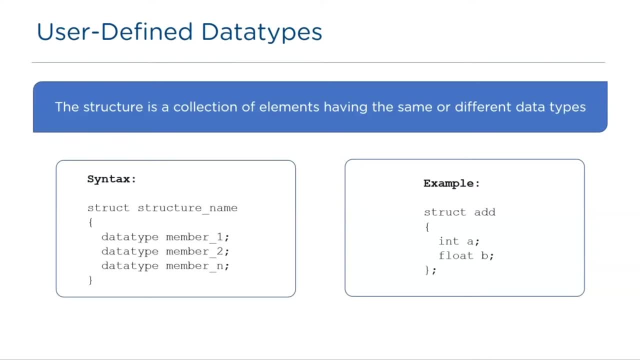 A variable. a is of type int and b is of type float. And finally, we have a union datatype that holds the different datatype elements in the same memory location. In the following example, the union is a keyword. Followed by that, we have a union name. 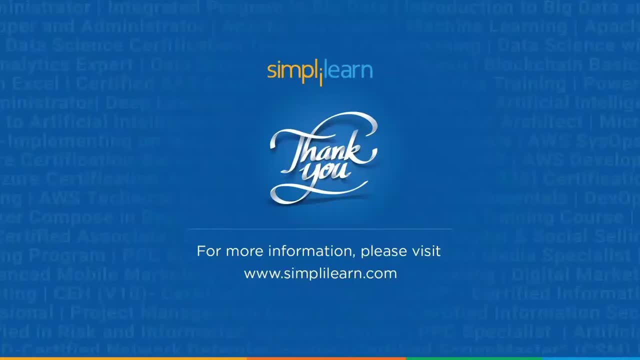 And then the variable list. So with this we have come to the end of this session on the datatypes in C programming. I hope this session was informative and interesting. Until next time, thank you, stay safe and keep learning. Hi there.